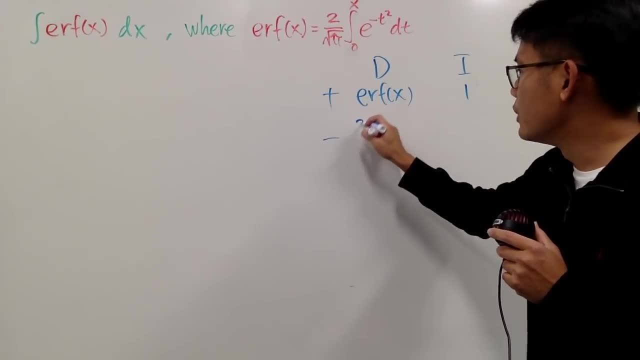 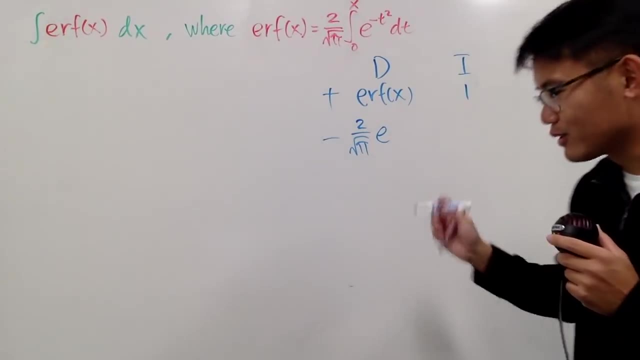 That's pretty much it, And this is the constant multiple. So I'll just write this down: 2 over square root of pi times no more integral, because the derivative and integral cancel each other out pretty much. and put the x right here, So you have e to the negative x. 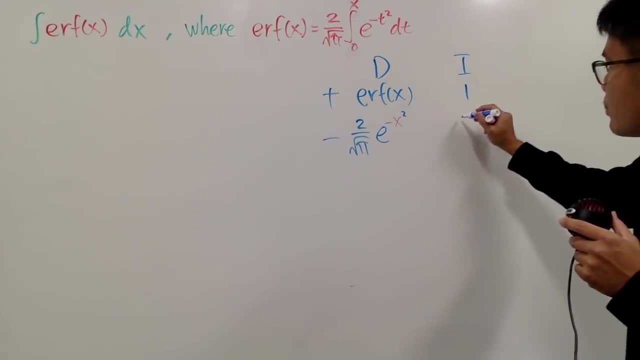 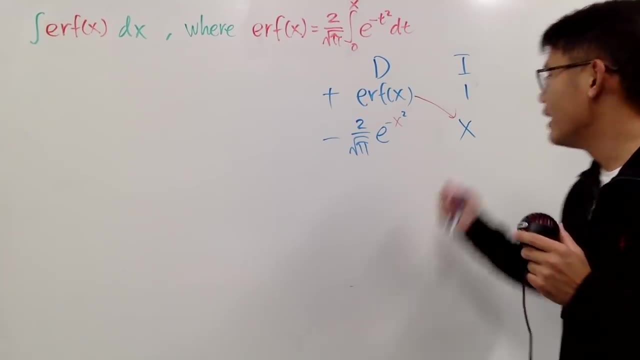 Square, And that's it. And to integrate one, you just pretty much get x, And now, of course, we can just go ahead and do this times this, And that will be the first part of our answer. Let me write down the x first, though. 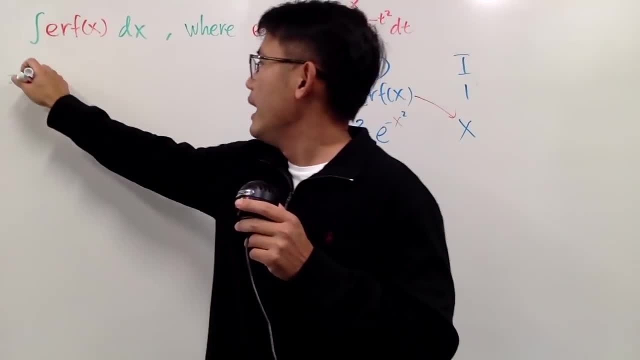 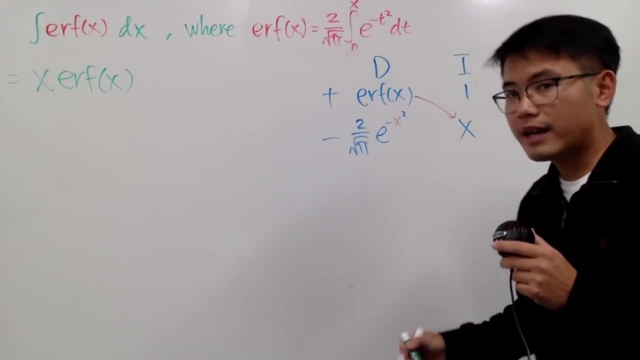 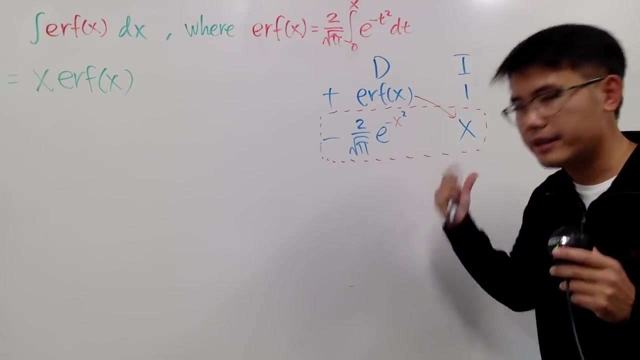 So we are talking about this is equal to x times erf of x. And then for the second integral, don't forget that we look at this row right And this right here, It's still an integral, The product of this, it's still an integral. 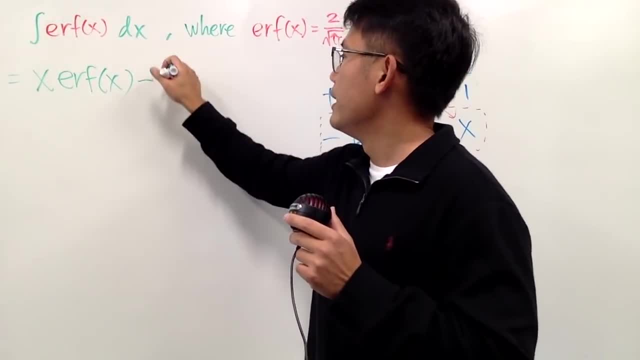 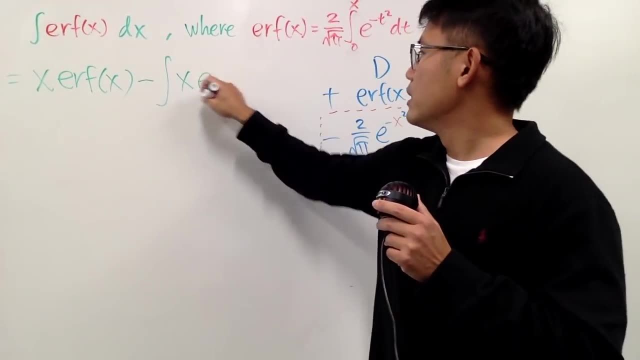 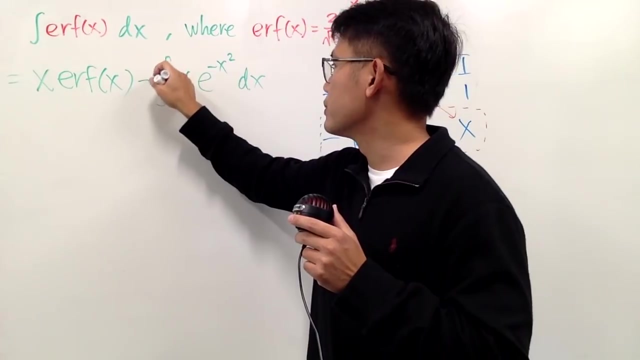 And this is a minus, So it's negative. Let me just write that down: Integral, And of course I can put down the x right here. And then we have the e to the negative x square dx. And since this is just a constant multiple, let me put that in the front, which is 2 over square root of pi, like that: 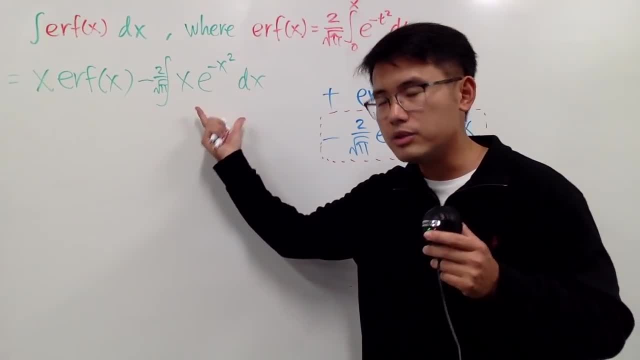 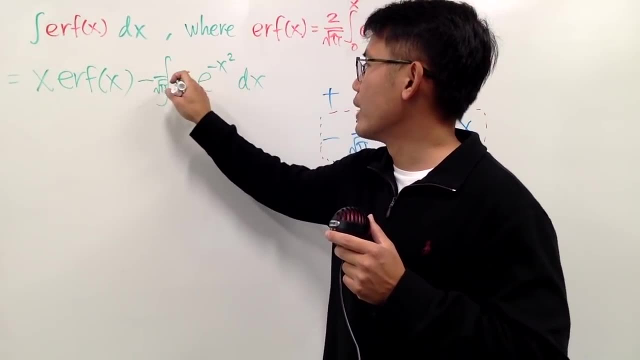 And in fact, depends on how you want to do it. You can just do this in your head. pretty much. This is totally doable now, right? So if you look at this, if you put a 2 right here, instead you have one like this: 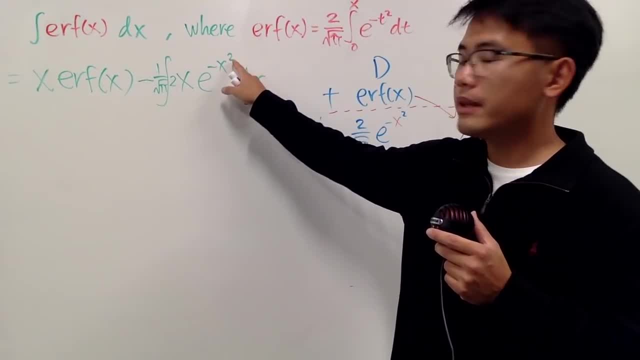 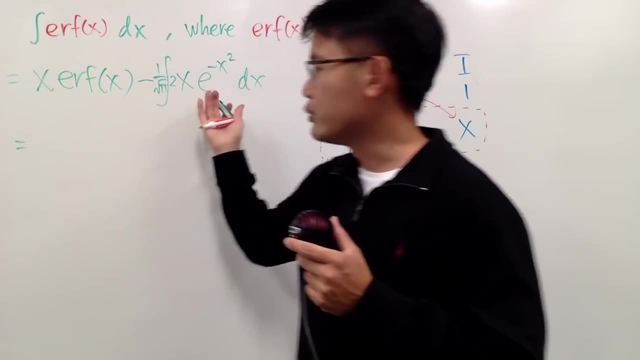 You see, the derivative of negative x square is negative 2x. In fact, you have the negative 2x right here as well. So, all in all, you pretty much can just do this by u sub letting u equal to negative x square. 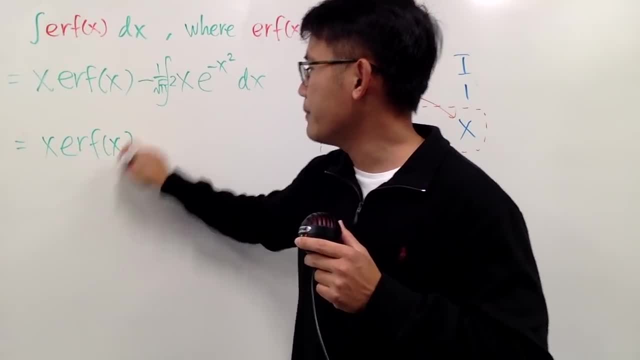 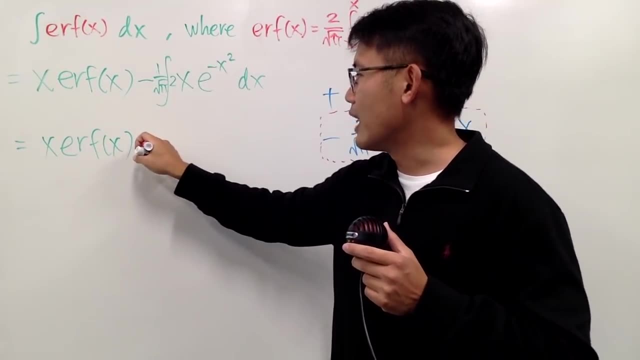 And the first part of the answer stays the same. So let me just write that down. But this is going to be cancelled after you do the? u sub. So you're pretty Pretty much. you have this part by itself, So you have plus, right. 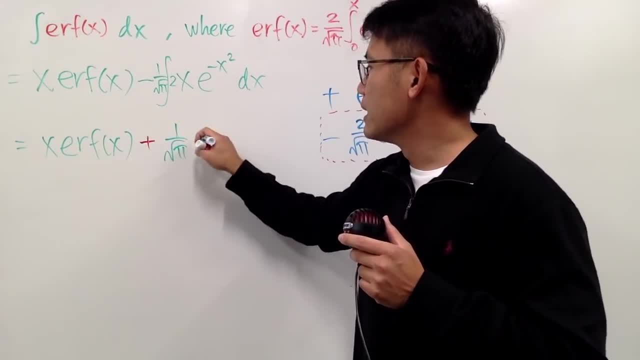 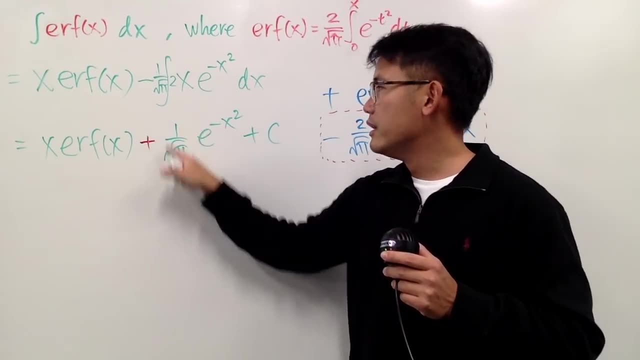 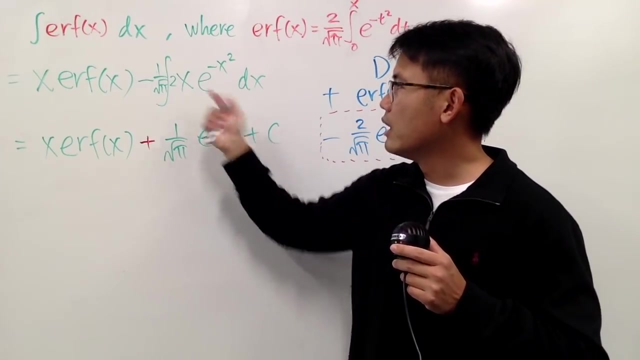 And then you have that 1 over square root of pi, e to the negative x square, Just like that, And we are done. And once again, if you differentiate this guy, this right here stays, And then this right here stays. But the chain rule says we have to multiply by the derivative of negative x square, which is negative 2x, right here. 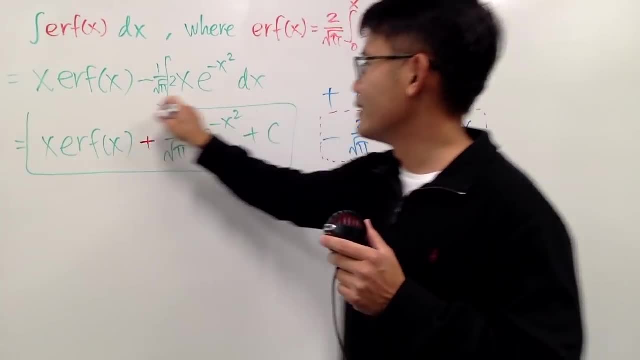